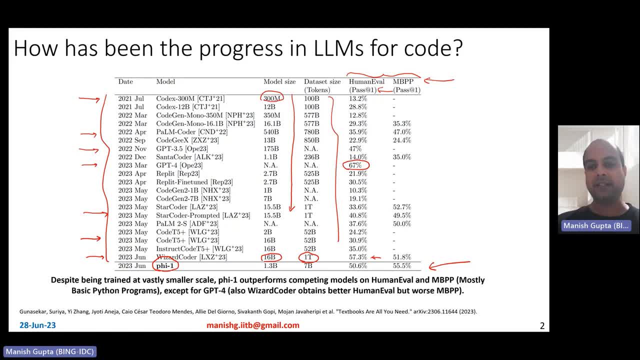 On the other hand, for the MBPB task, MBPB data set, essentially, again, you know, there have been good progress around 52.7 is more or less like the best result for that model, best evaluated result for that model. Now, the 5.1 model that we will discuss in this paper. Essentially, it's sort of close to these best results. So 52.755. So, in fact, for MBPB data set, it is actually one of the best models. For human-eval, it is not as good as GPT-4 for, you know, for sure. However, you know, if you look at the model size, it's just 1.3 billion, right? Very small sized model. Very, very small sized model. 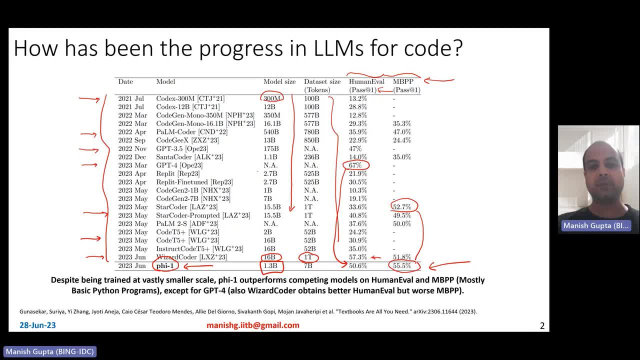 The closest model that you see around 1.3 billion is this 2.7 billion model. But then it has... 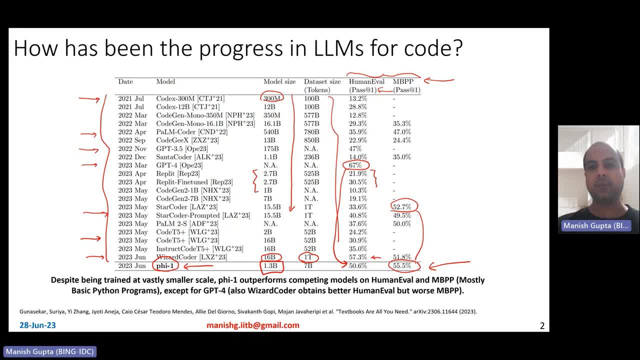 It has very poor performance in terms of human-eval or, you know, human-eval compared to the performance that you get with the 5.1 model. 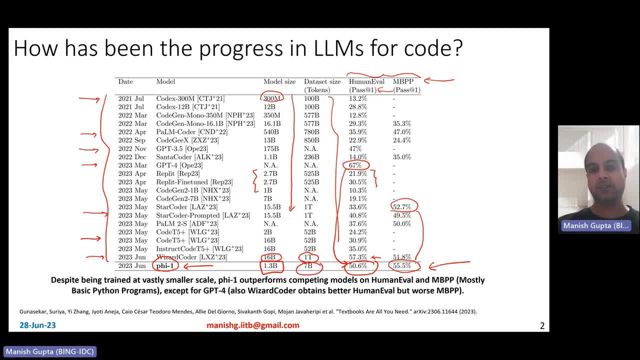 Also, the training is super cheap. It has been done using just 7 billion tokens. So the training data is actually very, very small. 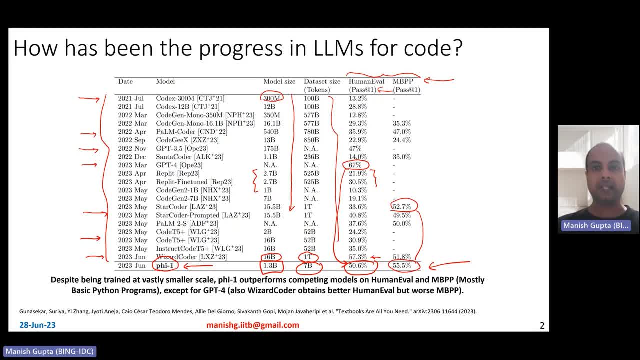 And all this is possible because of very high quality data that has been used to train this particular 5.1 model. So this leads me to this question, how important is training with high quality data? 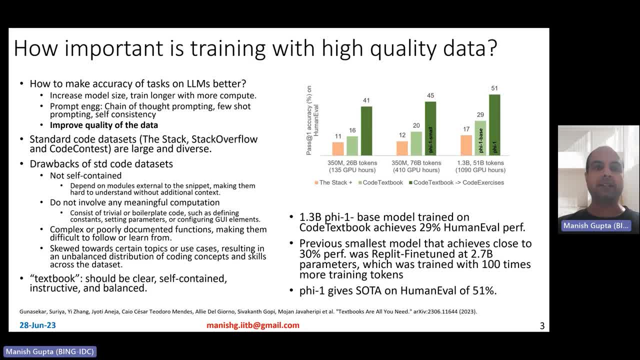 So, now, I think an important follow-up question. 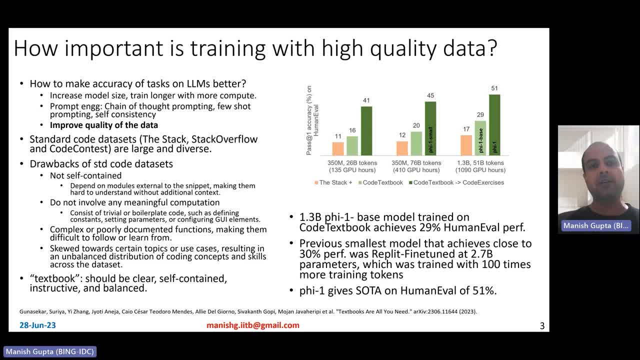 Or a reason why this question is important is the following. How to make accuracy of tasks on LLMs better? 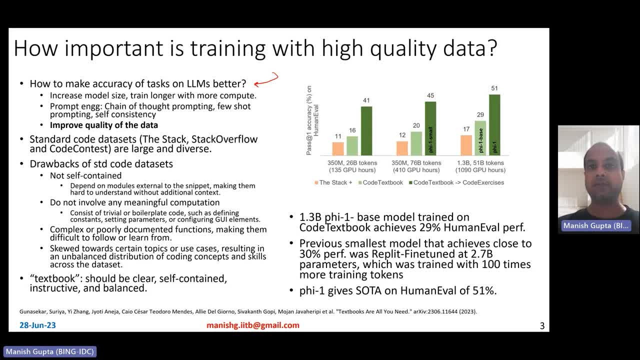 How to make LLMs, large language models, even more accurate on various kinds of tasks? So people have experimented with various kinds of methods. The most popular ones being increasing the model size or training longer with more compute. So, of course, what has also become popular these days is prompt engineering. So you can do chain-of-thought prompting, few-shot prompting, self-consistency, and so on, just to actually get better and better accuracy. 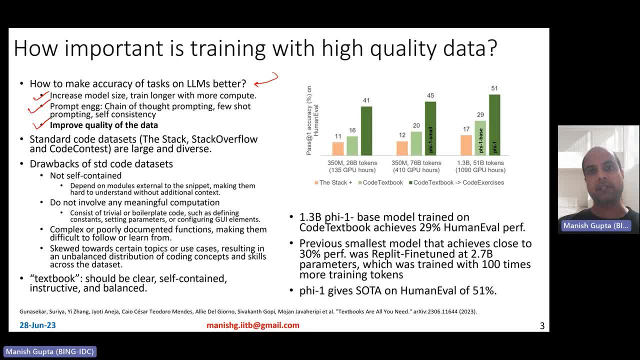 Yet another way of improving accuracy is improving the quality of the data, of the data which is used to pre-train and fine-tune these large language models. 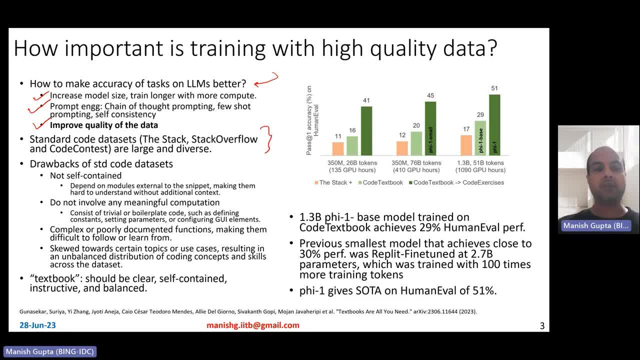 So for code, standard code datasets include the stack and stack overflow and code contest. So these are large datasets, and they also have very diverse code bases. 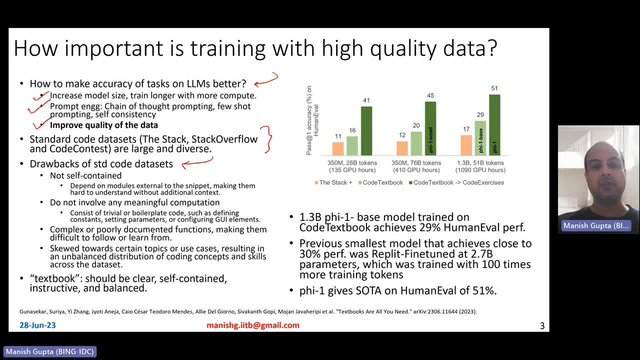 Now, the drawbacks of these standard code bases, standard code datasets are as follows. They're not self-contained. Many of the files inside these code datasets, many of the samples are not self-contained. Meaning, many of them sort of depend on modules which are external to the snippet. 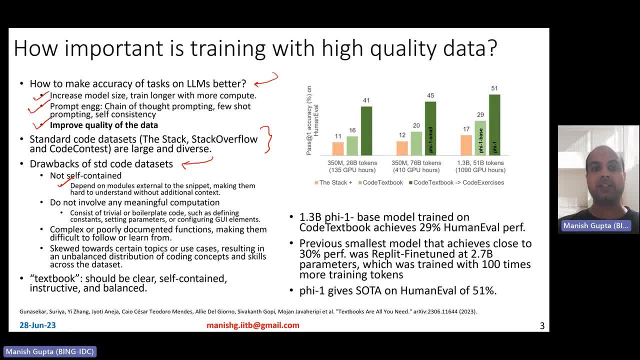 And therefore, it is very difficult to incorporate that additional context when you're training a large language model on these samples. Many of the samples in these standard code datasets do not involve any meaningful computation. They consist of, basically, I mean that they consist of trivial boilerplate code, such as defining constants, setting parameters, configuring GUI elements, and so on. Now, oftentimes, they include complex or poorly documented code. Now, oftentimes, they include complex or poorly documented functions when those functions capture deep algorithms, right? So making them difficult to follow or learn from them. 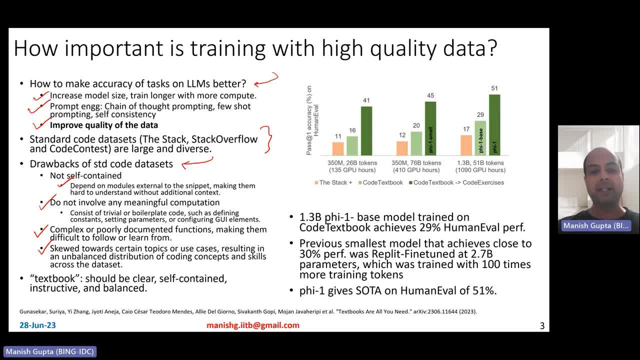 They're also skewed towards certain topics or use cases, resulting in an unbalanced distribution of coding concepts and skills across the entire dataset. 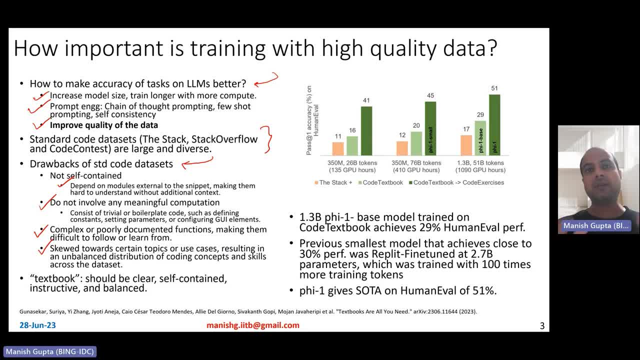 But if you were to have a kid learn how to code, you would rather want something which looks like a textbook, which should be clear, concise, self-contained, instructive, and balanced, right? 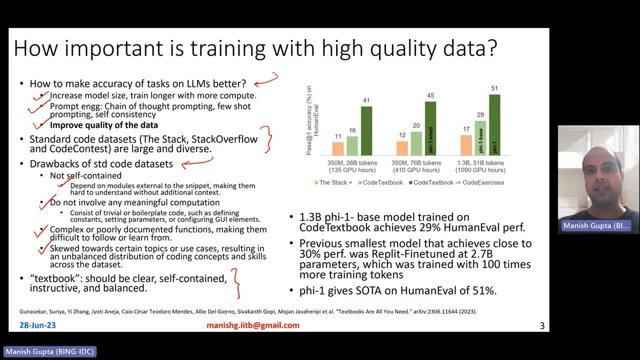 If you have that kind of a textbook, the kid learns well. 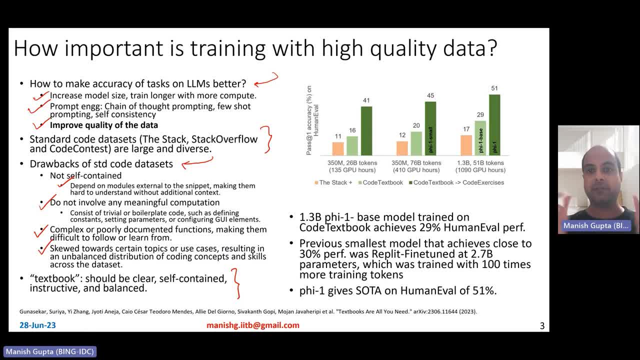 And the samples can also be expected to train well if you train on such textbook kind of data, which is what is observed in this paper while training the 5.1 model. The 5.1 model is a 1.3 billion parameter model. 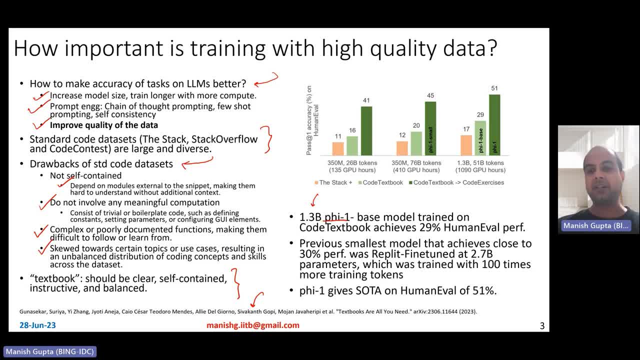 The 5.1 base model, specifically, has been trained on code textbook, and it achieves 29% on human eval performance. 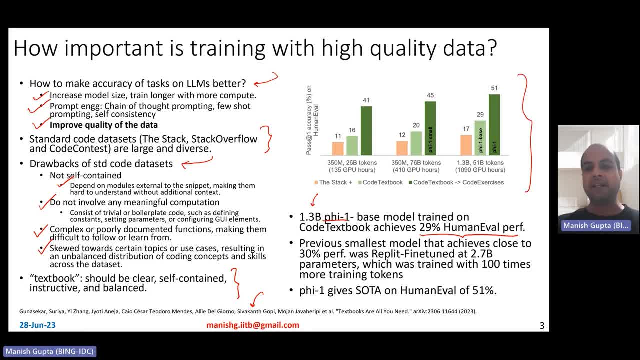 So, you know, the results are shown in more detail in this chart, where there are three different models being compared. 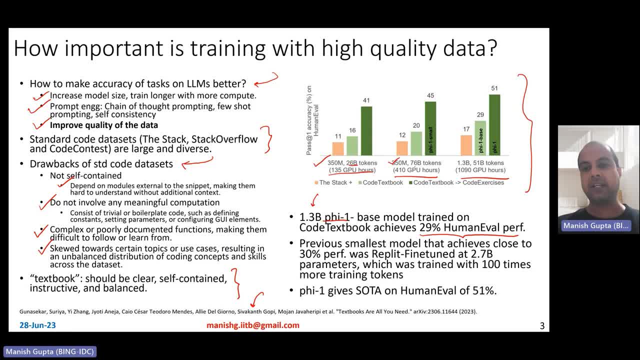 The 350 million model, which has been trained for 26 billion tokens. 350 million model trained for 76 billion tokens. And 1.3 million model trained for 51 billion tokens. 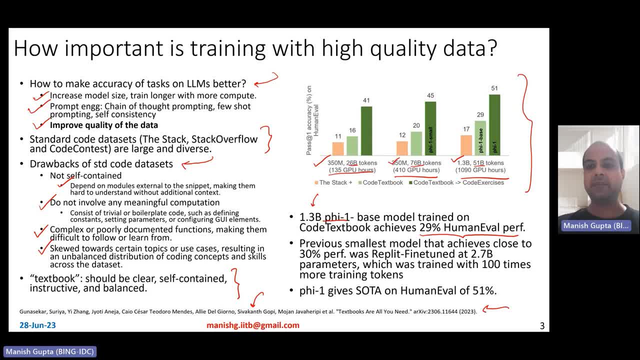 In this paper, there are three models which are specifically named. So, for example, this one is called 5.1 small, this one 5.1 base, and this one is 5.1. 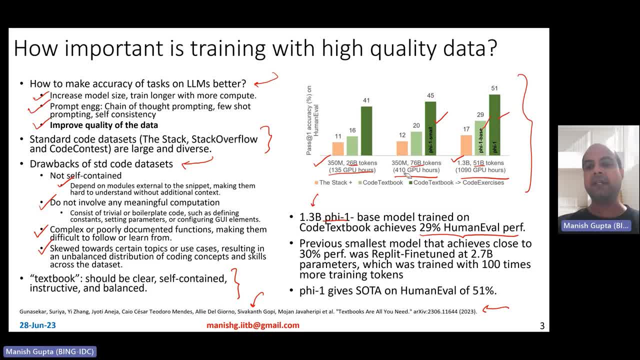 So 5.1 small is a 350 million parameter model, but it has been trained using 76 billion tokens. 5.1 base is a pre-trained model, in some ways, a 1.3 billion pre-trained model. 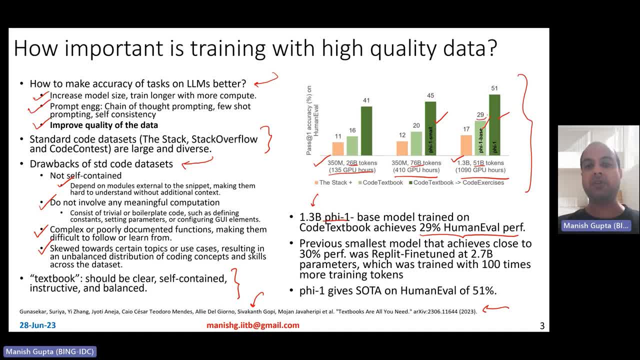 And the nice part is that it's not just a pre-trained model. The nice part is that it can actually achieve around 27% pass-at-one accuracy on human eval. 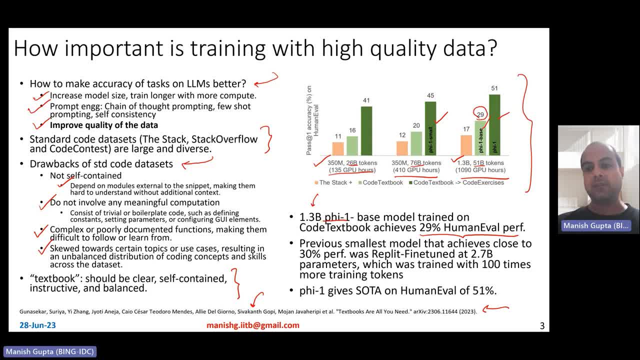 Now, an interesting point to sort of note is that if you train on standard data sets like the stack, stack overflow, and so on, you can only achieve so much of pass-at-one accuracy across different model sizes and model compute power, right? 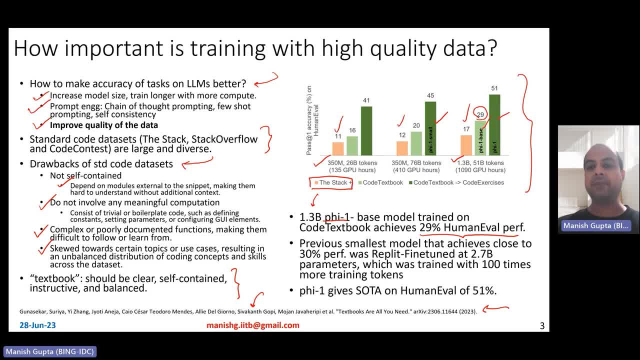 However, if you basically start training on, you know, on code textbook, and code exercises, which are cleaned versions of code data sets, you actually suddenly, you know, see that the accuracy improves across all different model sizes. 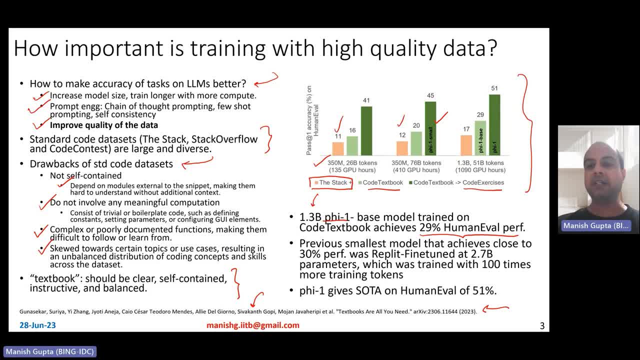 So, for example, if you basically not just pre-train on the code textbook data, but also further fine-tune on the code exercise data, you observe that the 5.1 model actually has a very high performance of 51%. Okay. So that's that. So how is 5.1 trained? How is the 5.1 model trained? 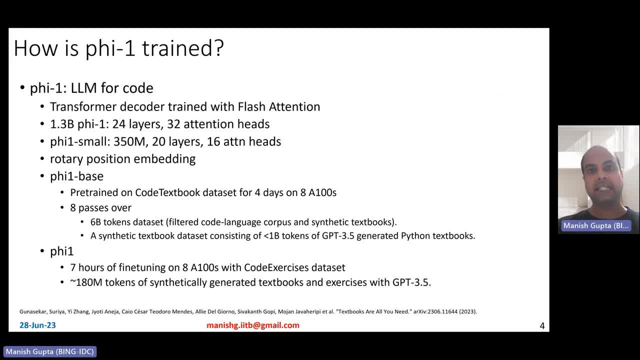 5.1 model is a LLM4 code. It is a transformer decoder trained with flash attention. 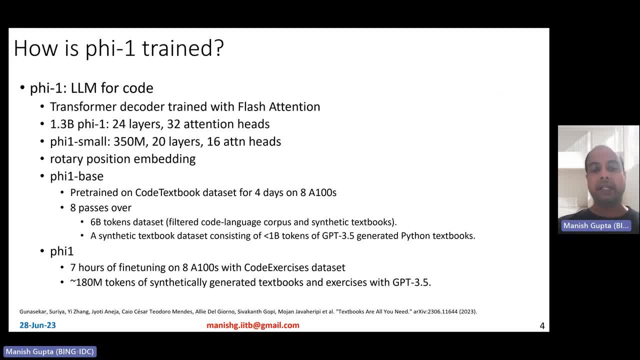 So it is trained using deep speed on eight 800 GPUs. 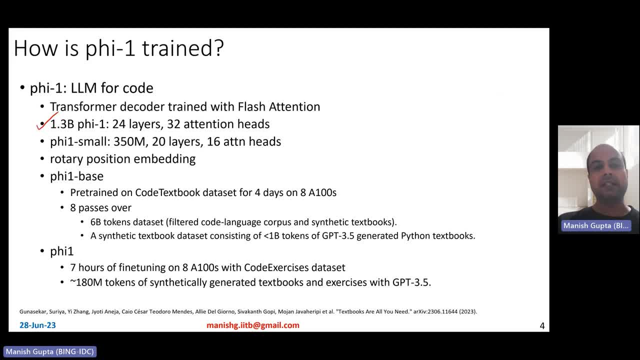 1.3 billion parameter 5.1 model actually contains 24 layers and 32 attention heads. The smaller model, which is 350 million, a 5.1 small model, it contains 20 layers and 16 attention heads. Okay. Okay. Okay. Okay. Okay. Okay. So that's rotary position embedding. 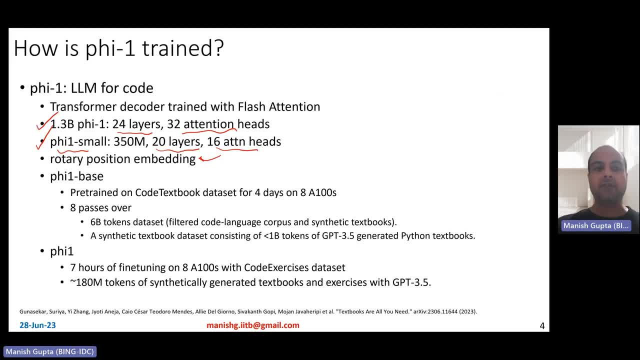 Now, a little bit about the 5.1 base and the 5.1 model. Well, 5.1 base and 5.1 model, both of them are 1.3 billion parameter models. 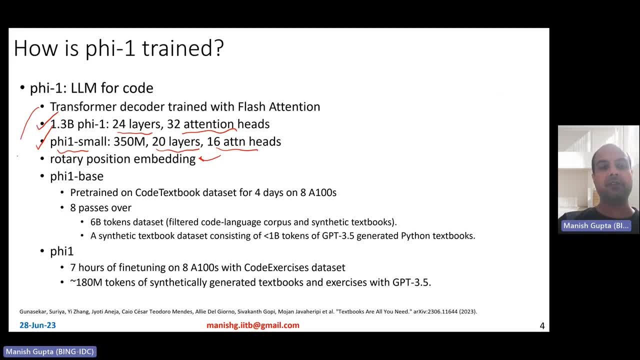 5.1 base is a pre-trained model. It is pre-trained, you know, from scratch, transformer decoder model. And it has been pre-trained using a data set called a code textbook data set. In the next few slides, I'll talk about how this code textbook data set is created. 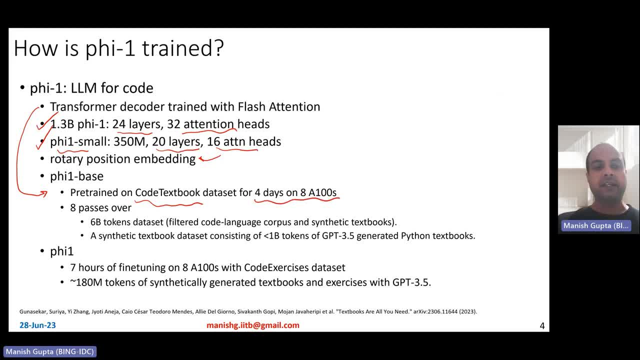 Okay. It has been trained for four days on eight 800s. That's a very small amount of compute power if you think about it, right? Just eight 800 machine is what you need in four days of that. And you can actually train a 5.1 base model. 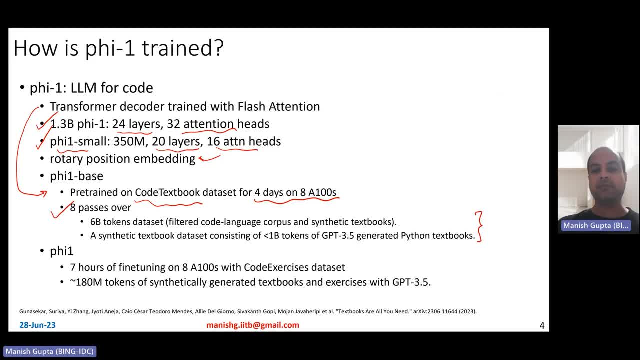 It does eight passes over this code textbook data set, which consists of these two parts. The first part is 6 billion token data set, which has been obtained by filtering code language corpus and synthetic textbooks. 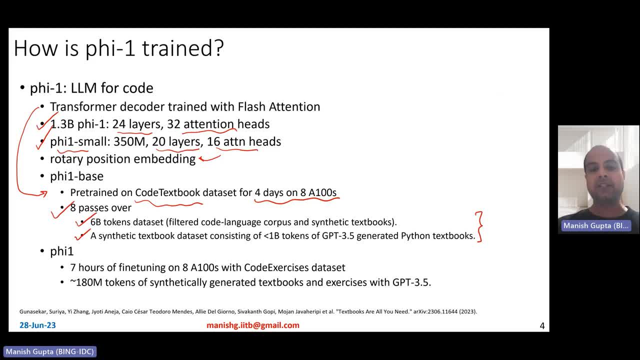 The second one is a completely synthetic textbook data set, which consists of less than 1 billion tokens. So overall, 7 billion tokens in this data set. 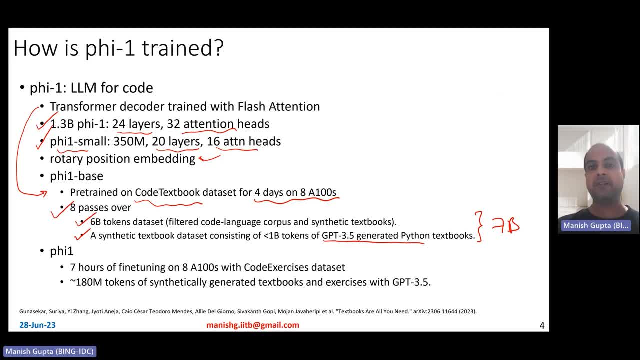 So the synthetic data set has been opened. It has been obtained using GPT 3.5. GPT 3.5 was used to generate Python textbooks, as we'll see soon in the next few slides. Okay. So that's the pre-training part. 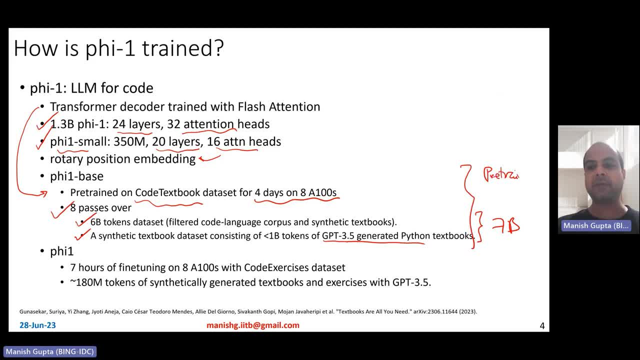 This is the pre-training part using which, you know, 5.1 base model has been pre-trained. Now, the second part is the fine-training part, which is how the 5.1 model has been trained using the 5.1 base model. 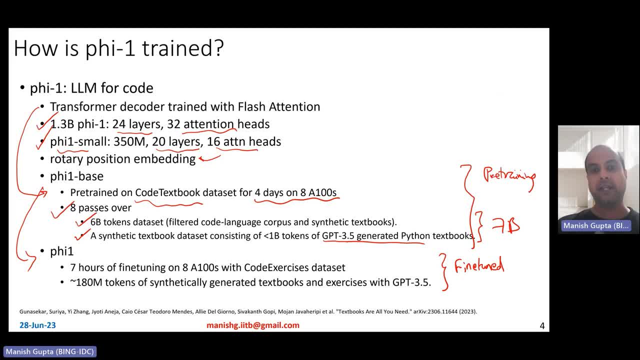 It basically just requires seven hours of fine-training. That's it, on the same eight 800 machines with codexized data. 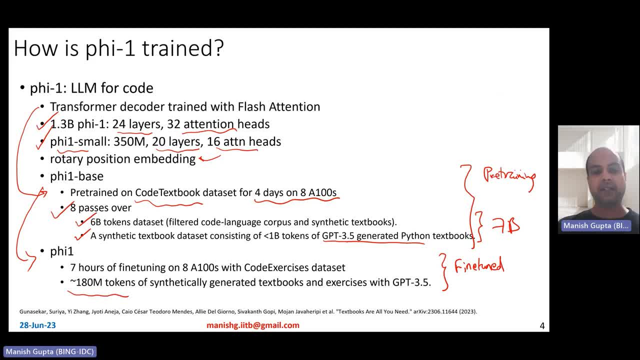 Now, codexized data. Again, a very small data. It contains 180 million tokens of synthetically generated textbooks and exercises, again, using GPT 3.5. 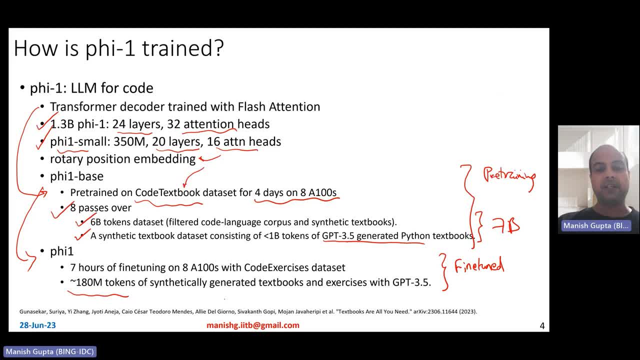 We will quickly talk about how the code textbook data is obtained, how codexized data is obtained, and also how this filtering of the code language corpus is done in the next few slides. 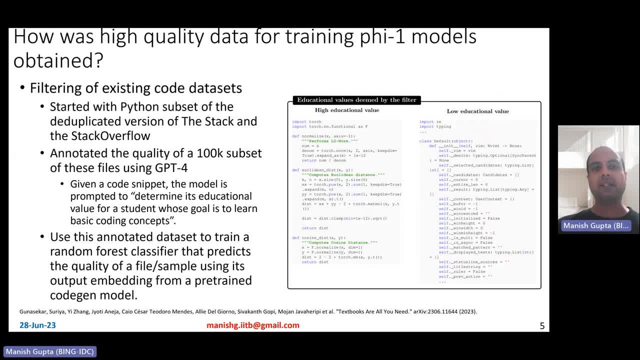 So how was high-quality data obtained for training 5.1 models? Well, the first step is to filter existing code data sets. 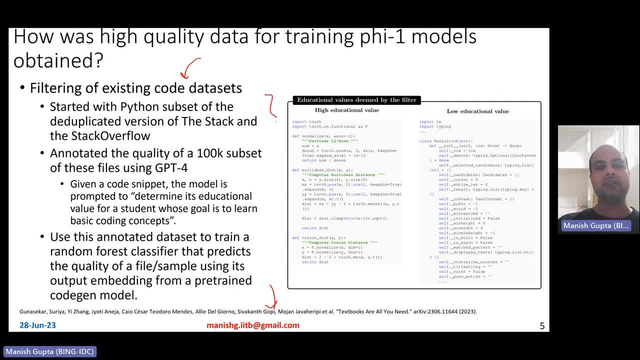 So the authors actually started with Python. Python is a very common subset of the deduplicated version of the stack and stack overflow. 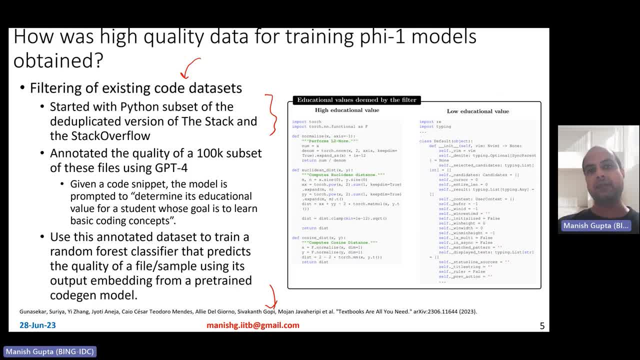 So that's the original base data. These, you know, billions of such files were actually, or billions of these tokens in these files were annotated for quality using GPT-4. 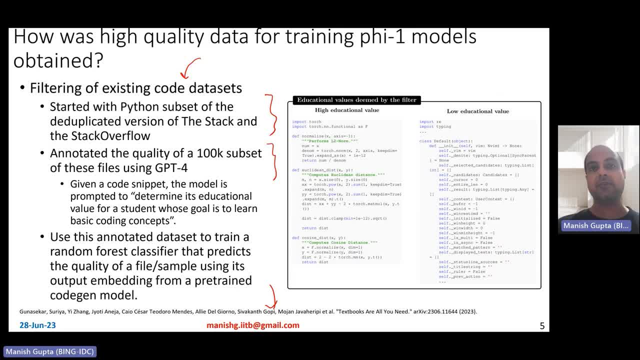 Not all of them, just 100k subset of these large number of files were annotated using GPT-4 for quality. 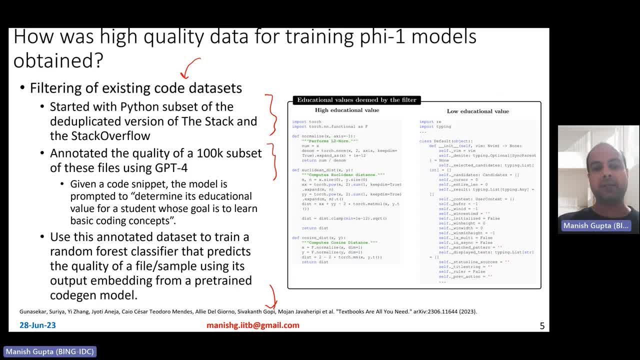 Given a code snippet, GPT-4 was basically prompted to determine its educational values. 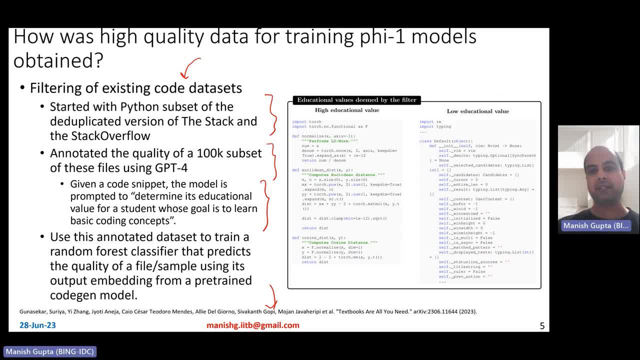 So for example, this particular first part of the code basically would be labeled as high educational value because, well, it basically tells you how to perform L2 norm, how to compute Euclidean distance with appropriate commands and so on. 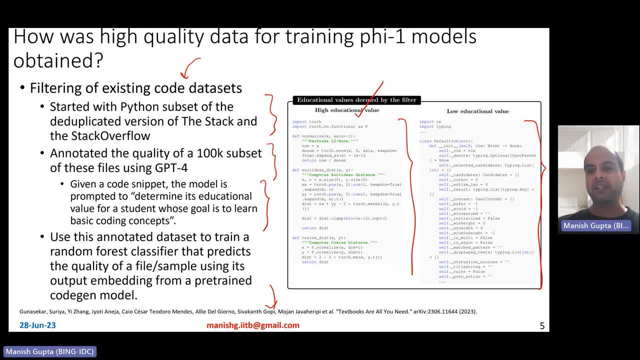 While this is going to be called as low educational value because if you see, it sort of looks like more like templatized code, boilerplate code, which basically is just doing self-taught. So setting some properties, that's it, rather than actually teaching. 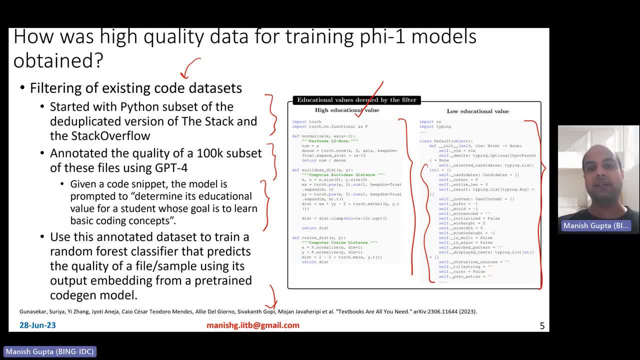 How certain functionality can be used, let's say, in a Torch, like in the Torch library. So using this small 100k subset of labeled data from GPT-4, the authors actually trained a random forest classifier that predicts the quality of a file or a sample using the output embedding from a pre-trained CodeGen model. That was the first part of obtaining the code textbook data. 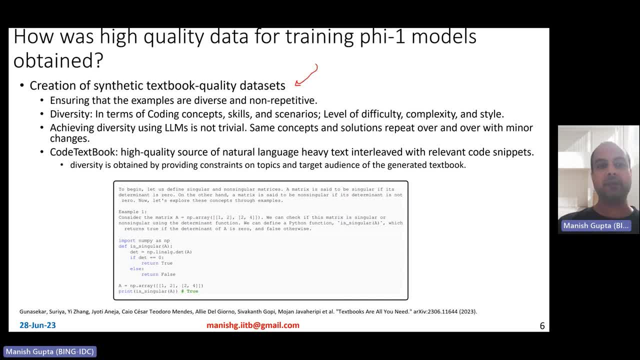 The second part of code textbook data is actually obtained synthetically using GPT-3.5. So the idea was to integrate the code textbook data into the GPT-3.5. 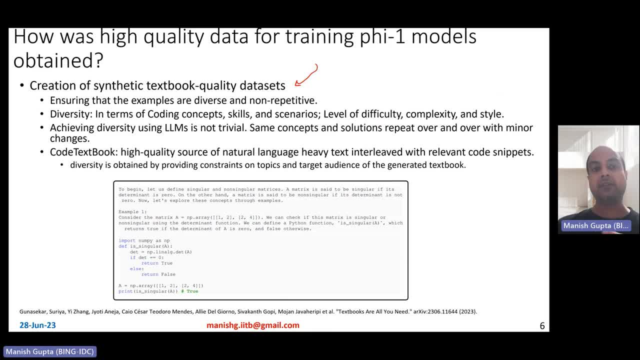 to ensure that the examples generated by GPT-3.5 should be diverse and non-repetitive. 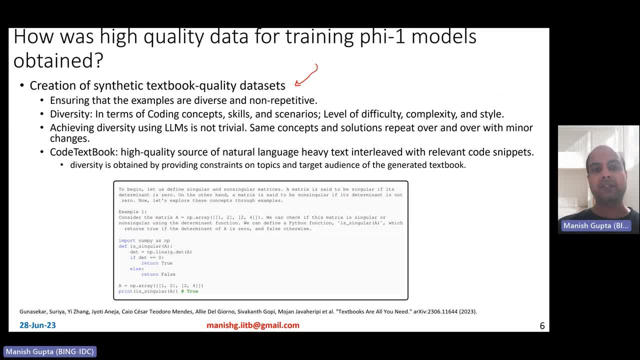 Now, by diversity, we basically mean that it should be diverse in terms of coding concepts, skills, and scenarios. 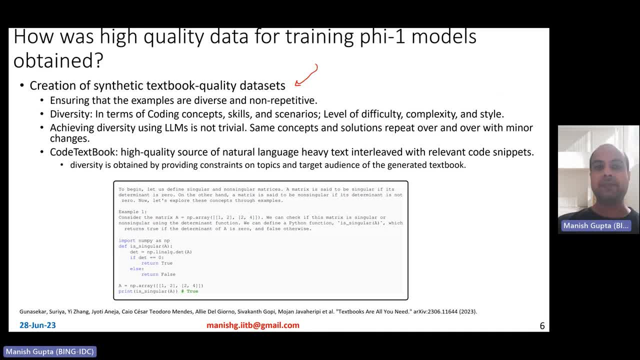 It should also be diverse in terms of level of difficulty of problems and examples, and also complexity and style of the examples. 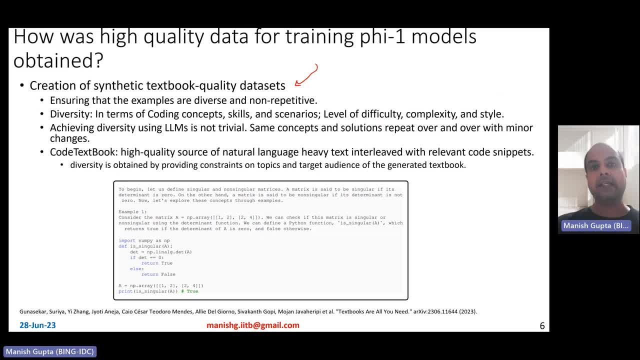 However, achieving diversity using GPT-3.5 or for that matter, any LLM is non-trivial. LLMs typically tend to repeat the same concepts and solutions over and over again. 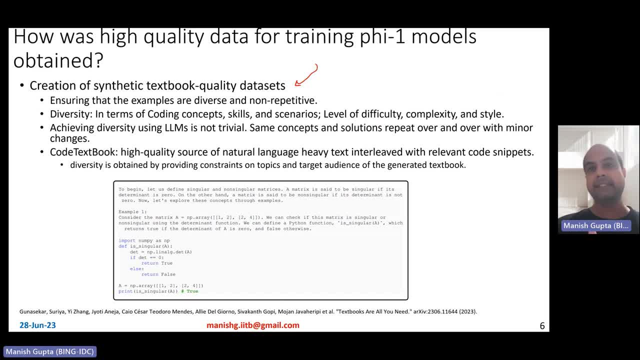 over again with minor changes if there are only small little changes that you do in the prompt 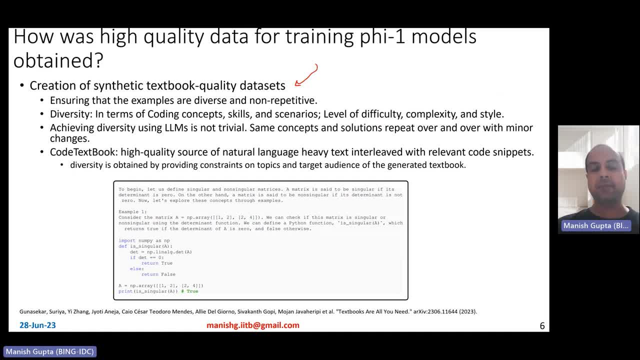 so how to basically obtain diverse you know examples from llms is complex so the way code 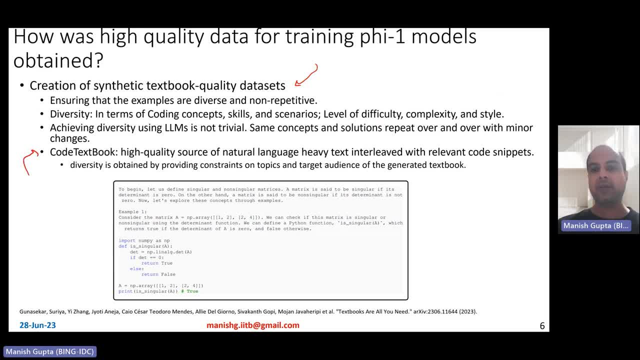 textbook data has been obtained well it's a high quality source of natural language heavy text 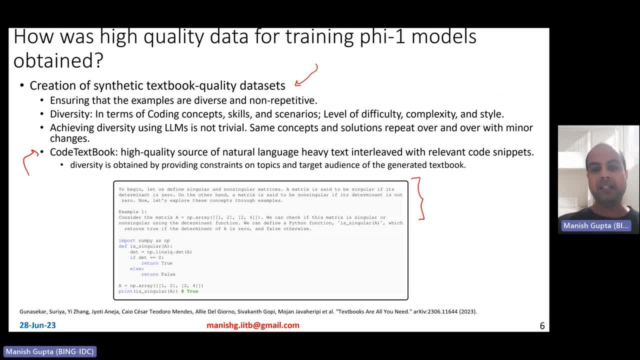 interleaved with relevant code snippet so there is text part which describes what is going on and 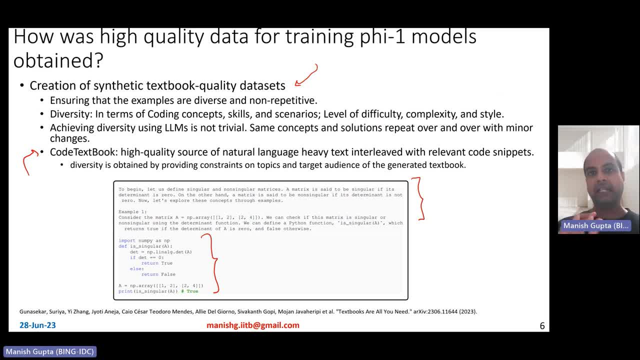 there is an example and then there is also code part so there is interleaving of text and code 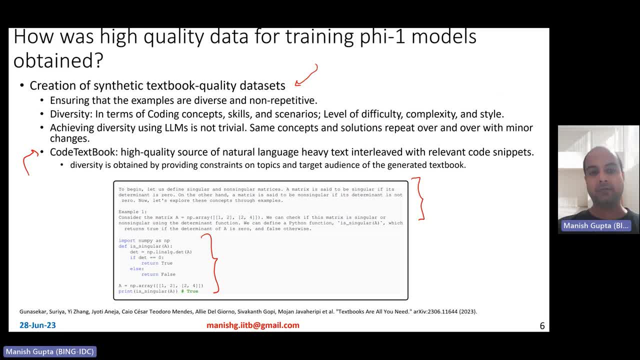 and well diversity is obtained here by providing constraints on topics on which the text and the 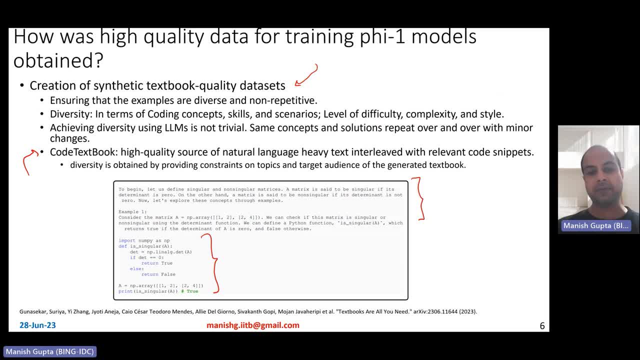 code should be written and the target audience of the generated textbook so that's that now the 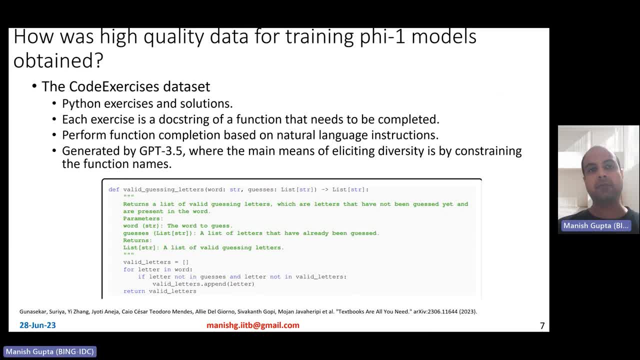 third part or rather the fine-tuning data set for phi1 model is the code exercise data set this data 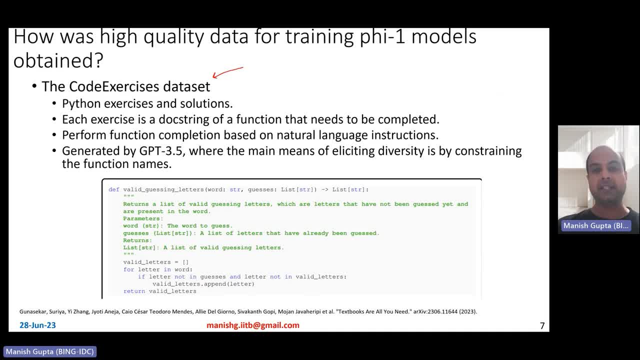 set consists of python exercise and solutions each exercise is basically a doc string of a function 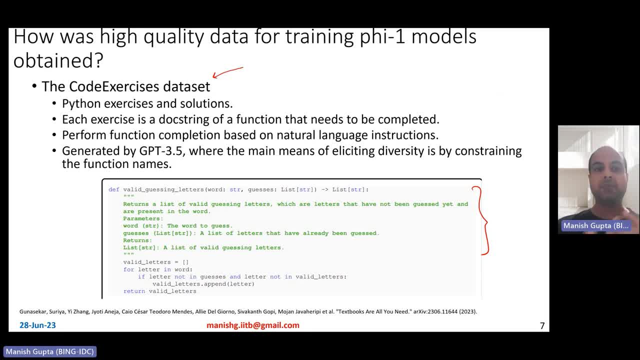 that needs to be completed in fact the gpt 3.5 model was prompted to perform function completion based on the natural language of the code so the gpt 3.5 model was prompted to perform function completion based on the natural language of the code so the gpt 3.5 model was prompted to perform 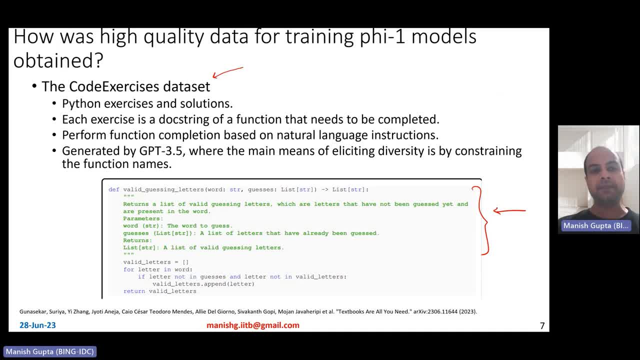 language instruction that was passed as part of the doc string right uh this the data has been 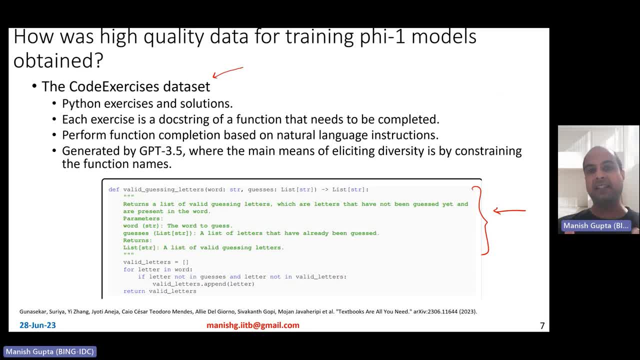 generated using gpt 3.5 where the main means of eliciting diversity is by considering the function 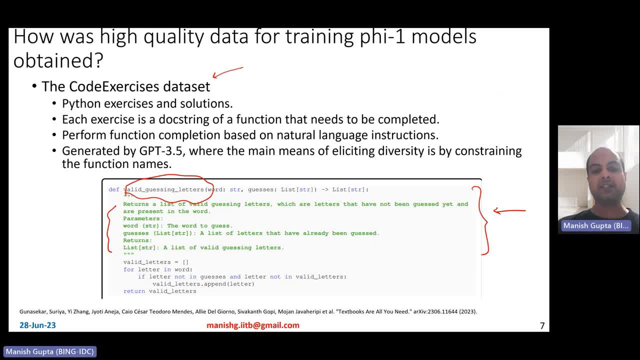 names so you basically give various function names and then give the doc string and you expect that the gpt 3.5 model will output interesting pieces of code so diverse pieces of code okay so we have 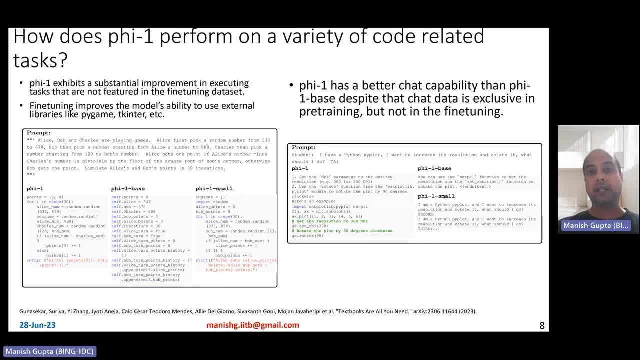 talked about how phi1 model has been trained and also we talked about how the high quality data for training phi1 model has been obtained now how does phi1 model perform on a variety of code related tasks right so interestingly it is observed that phi1 exhibits a substantial improvement in 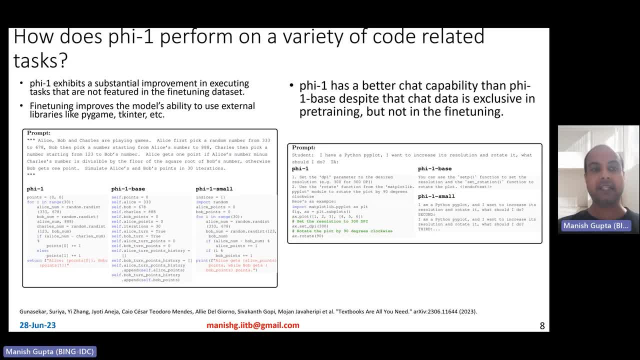 executing tasks that are not featured in the fine tuning task data set itself for example fine tuning improves the model's ability to use external libraries like pygame and kinter and many other libraries okay for example if you look at this prompt you know ellis bob and charles are playing 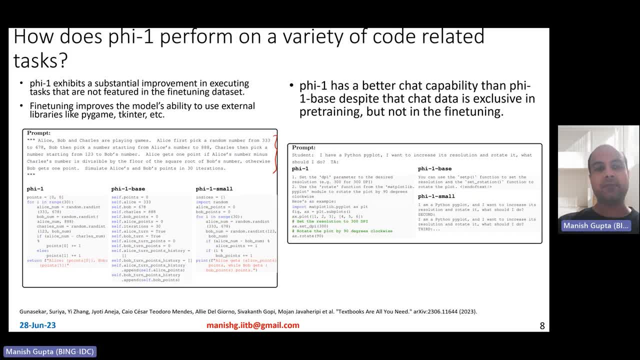 games um ellis first picks a random number from 333 to 678 bob then picks a number starting from ellis's number to 888 charles then picks a number starting from 123 to bob's number and so on so forth so as you observe the phi1 model actually very nicely generates code which is perfectly 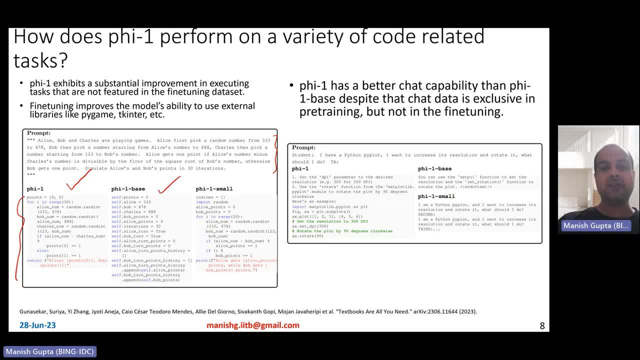 suitable perfectly correct code on the other hand if you look at the phi1 base model or phi1 small model well phi1 base model basically just is stuck in terms of defining some variables uh while you know phi1 small model does try to generate some reasonable kind of code however uh it also cannot generate very good co it doesn't end up generating correct code anyway 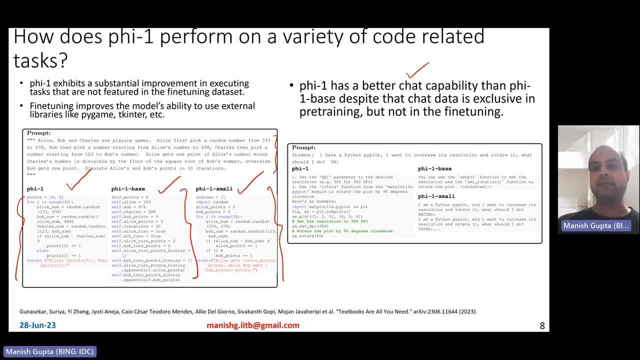 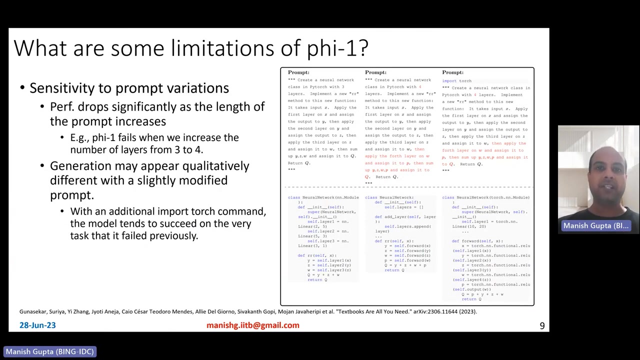 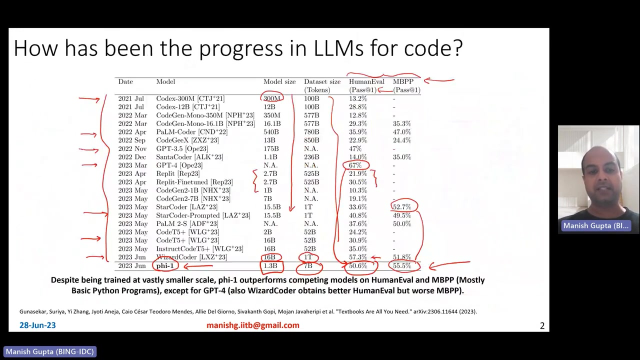 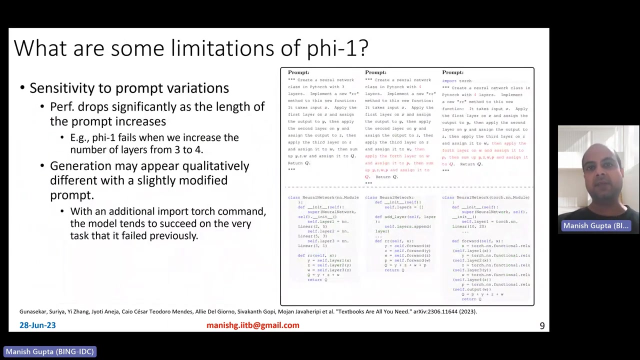 um phi1 also has a better chat capability uh than phi1 base model despite that the chat data is sort of exclusively used in pre-training part and not really in the in the fine tuning phase at all while phi1 phi1 base of course is the pre-trained version phi1 is the is the fine tuned version so here's an example uh prompt is basically a student saying i have a python pi plot i want to increase its resolution and rotate it what should i do so and then it the prompting is done as a t8 so you know expect the model to act as like a teaching assistant and answer and the model sort of generates a very awesome output first telling in terms of text what should be done and then also giving an example in terms of code that is how it is done okay so what are the limitations of phi1 model remember phi1 model is very small so compared to very large models like star code i'm not going to go into the details here but if you look at the model or the model of the model of the model of the model or or or you know various models that i mentioned in the beginning of this slideshow like wizard coder and so on um phi1 model is just 1.3 billion parameters compared to 10x plus parameters and it has also been trained on just 7 billion tokens compared to 52 billion tokens or even 1 trillion number of tokens that have been used for training other kinds of larger models right so given that 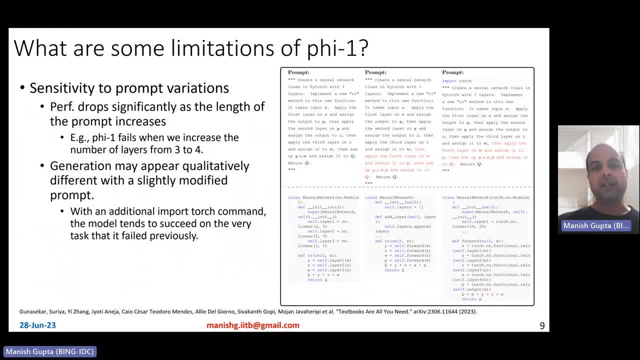 there are some limitations in the 5-1 model for example it is very sensitive to prompt variations performance drops significantly as the length of the prompt increases for example if you give a prompt so as to uh you know generate a neural network with three layers it does okay you know 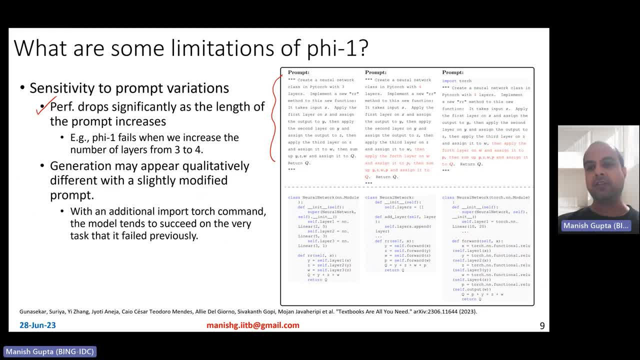 you basically uh tell it to sort of uh also add a fourth layer and well it just basically cannot perform that well phi1 fails when we increase the number of layers from three to four in that census 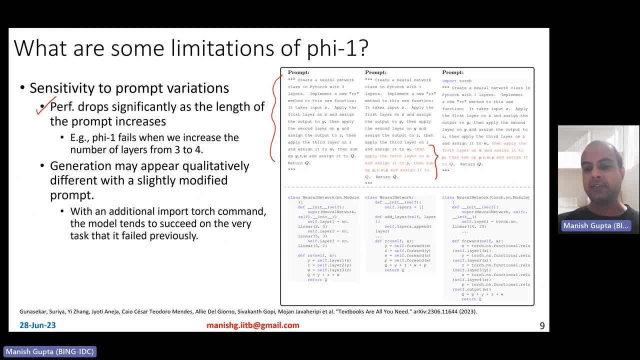 okay um you know uh and and you you see another example uh well uh i mean i'll talk also about this other example 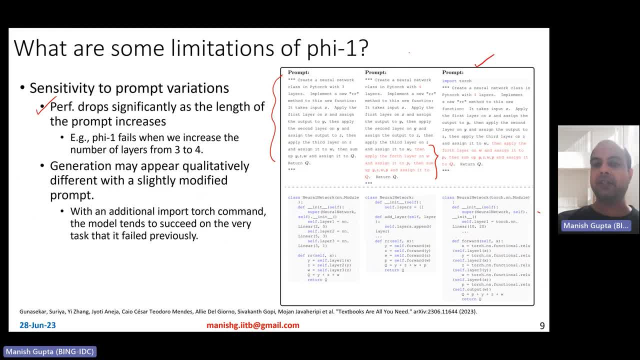 the idea here is that you know even though the network sort of the the phi1 model sort of feels in terms of generating a network with four layers but then you just in in you know include in the 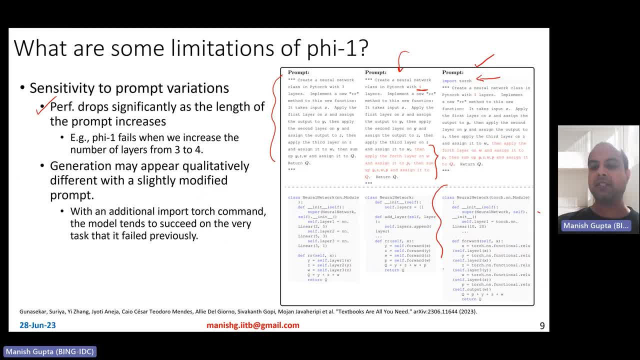 prompt this small little line import torch and everything somehow seems to work perfectly fine thereby saying that the model is pretty sensitive to prompt variations the generation may actually 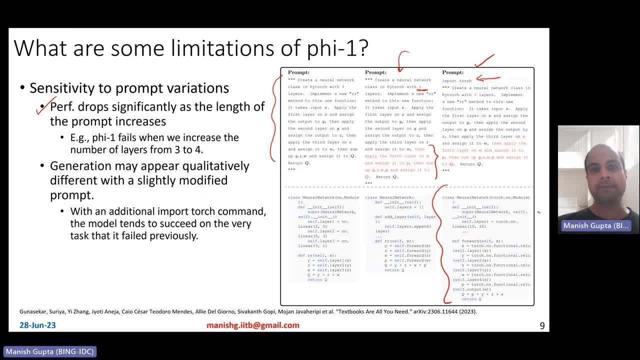 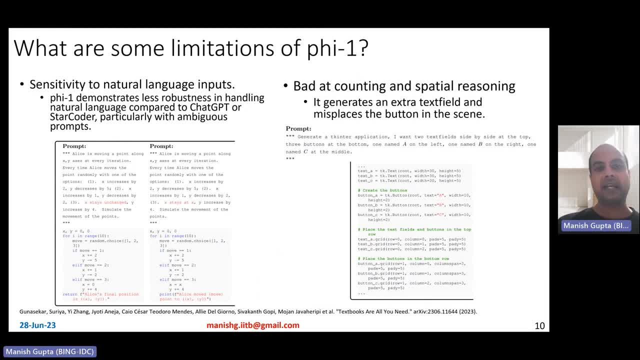 inputs phi1 sort of demonstrates less robustness in handling natural language compared to 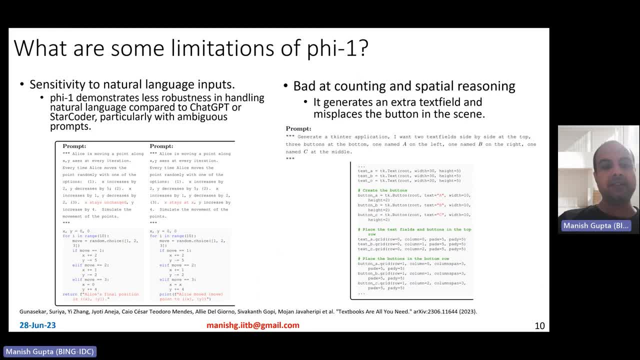 chat gpt or star coder kind of models for example here is here is a prompt example you say uh you know ls is moving a point along x y axis at every iteration every time ls moves the point randomly 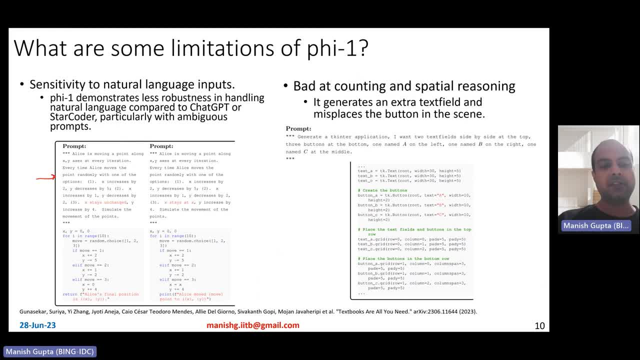 with one of the options one of these options these three options right so so this is good the code is good we are trying to choose one of three options and the first option says x increased by two degrees y degrees by five increased by two y degrees by five 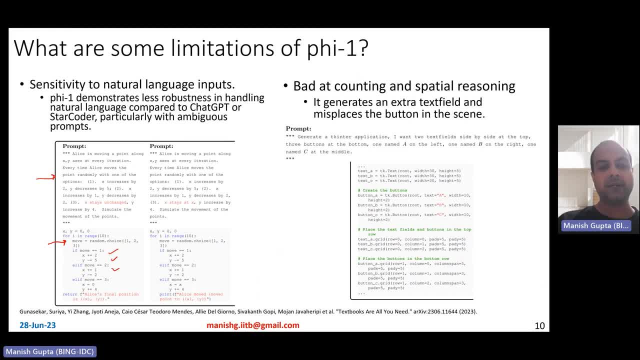 second option says x increases by 1, y decreases by 2, x increases by 1, y decreases by 2, that's okay, x stays unchanged, and the model somehow cannot understand this, so it basically says x 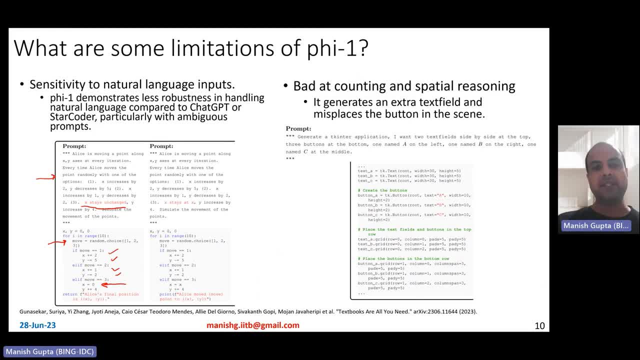 equal to 0, now x equal to 0 doesn't mean x stays unchanged, but then if you just change the wording a little, x stays at x, you know, it basically just performs perfectly fine, now of course 5.1 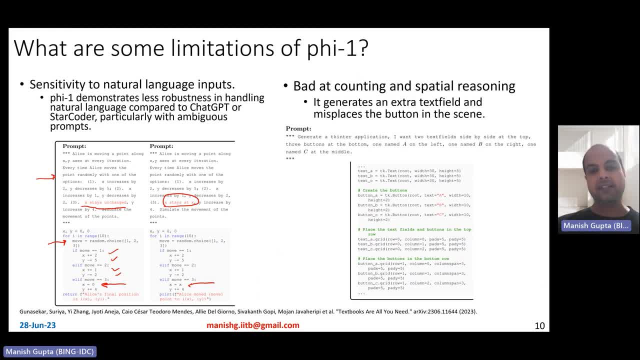 model has not been instruction fine-tuned in that sense, and therefore basically, you know, it does not really understand x stays unchanged that well, okay, 5.1 model is also bad at counting 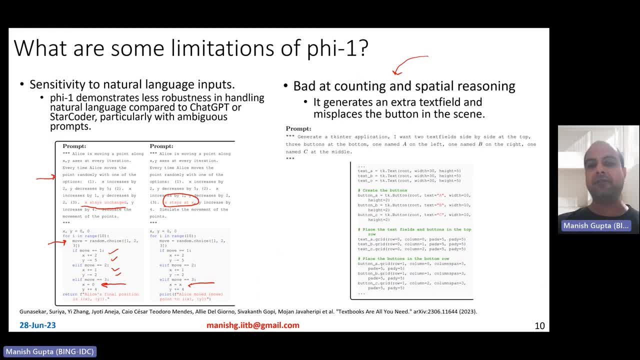 and spatial reasoning, so essentially, for example, if you basically create a application, you want two text fields, but then 5.1 model ends up basically adding three different text fields, 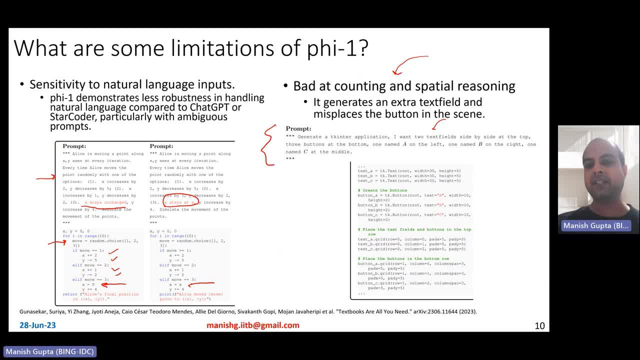 and, you know, you basically say, you know, three buttons at the bottom, it misplaces the button in the scene, right, when it creates the code in this application, okay.